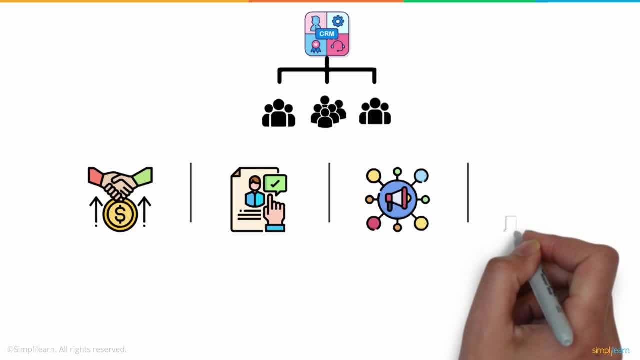 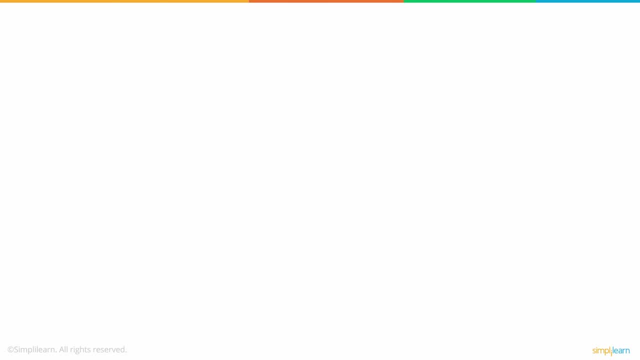 from sales and customer service to hiring, marketing and corporate development. A better approach to handling external interactions is the crux of CRM platforms. Joe, like Kevin, can use the CRM platform to centralize all customer data, track service issues, locate potential clients and manage marketing campaigns. 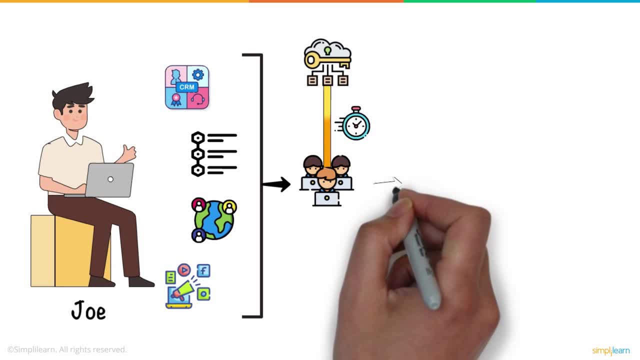 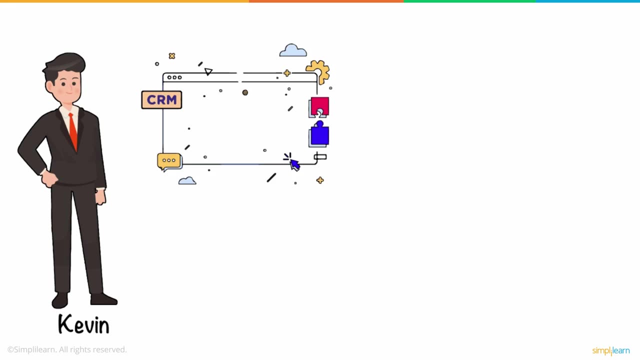 It will help Joe's team access data much faster and collaboration will become very smooth, leading to increased productivity. CRM platforms can serve companies of all sizes, from small start-ups to multinational corporations. Kevin's own start-up uses a CRM platform that utilizes cloud computing, also referred to as SaaS. 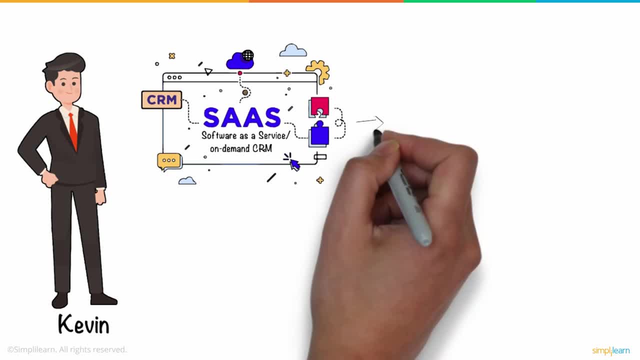 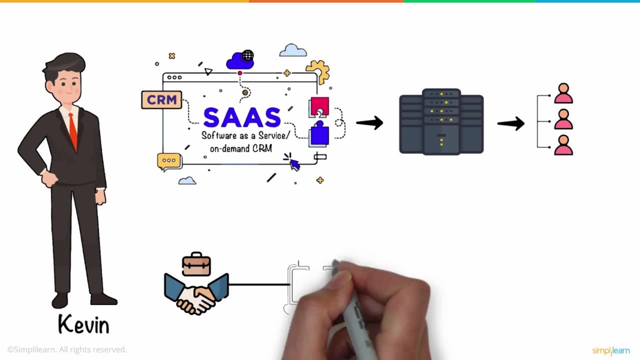 software as a service or on-the-go. Joe's CRM platform is designed to be able to access and manage CRM data on an external remote network that employees can access whenever they need to. Businesses with little technological know-how or resources are drawn to the cloud's speedy. 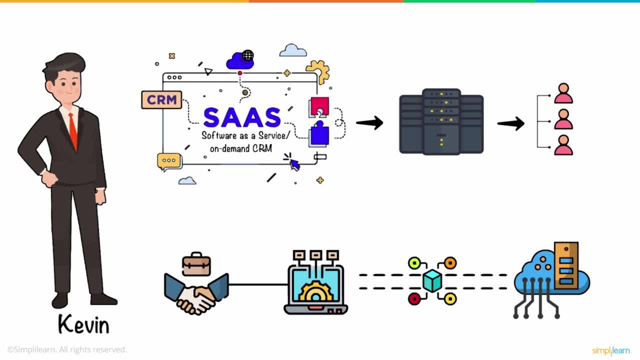 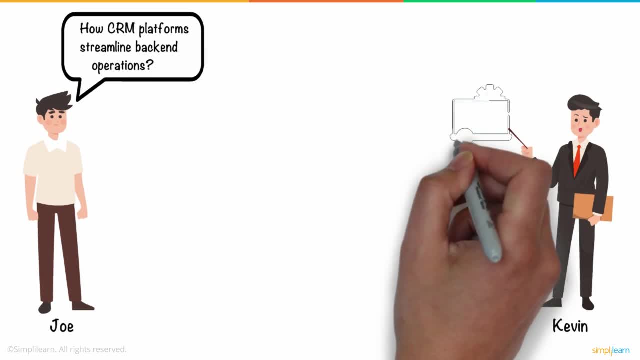 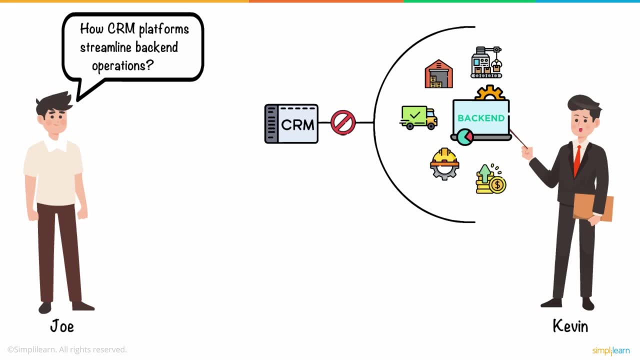 comparatively simple deployment possibilities. Joe wanted to know how CRM platforms streamline back-end operations, which Kevin clarified gladly. Back-end processes like manufacturing, warehousing, shipping, engineering or finance are not intended to be assisted by CRMs. Naturally, CRM technologies cannot control what they are unable to observe. 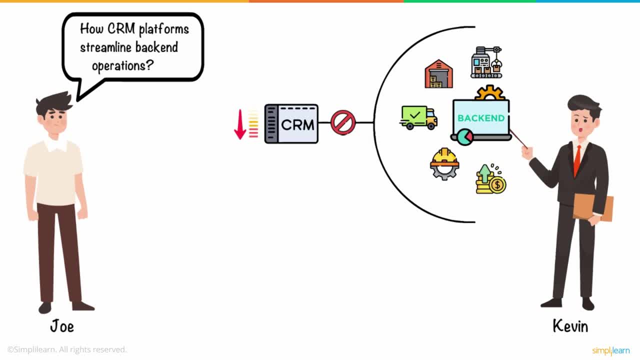 Therefore, it reduces the efficacy of the system for the entire team if employees work leads or transactions outside of it. Some CRM applications are simply used for data management to help entrepreneurs like Joe and Kevin run their complete business more successfully. An all-in-one CRM system. 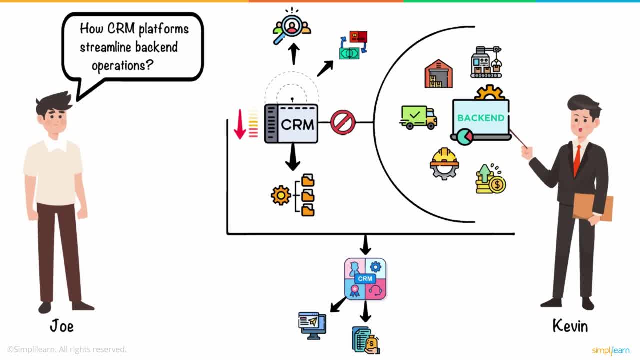 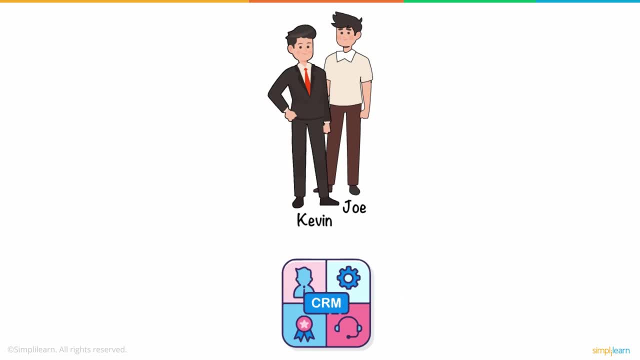 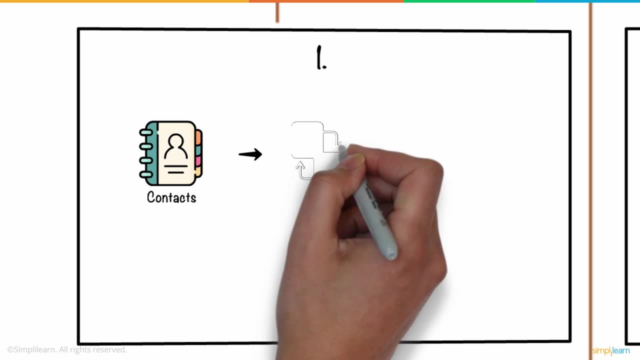 also provides crucial functions like landing pages, quotations and invoicing. Joe was still not convinced, Which led Kevin to explain how his startup benefits from their CRM platform. 1. All of Kevin's contacts are managed by a CRM, which also collects crucial customer data like 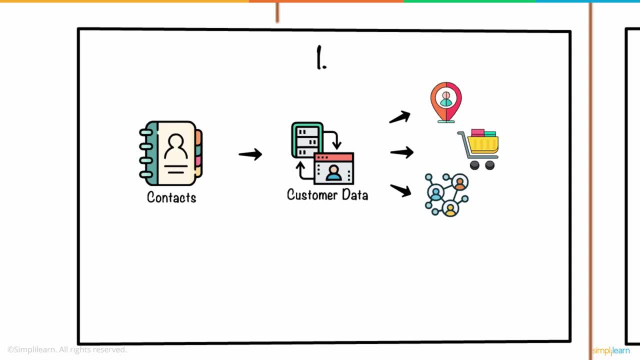 demographics, purchase histories and prior communications across all channels and makes it readily available to anybody in his organization who needs it. This guarantees that Kevin's staff has all the information they want about the client at their fingertips and can offer a better customer experience. 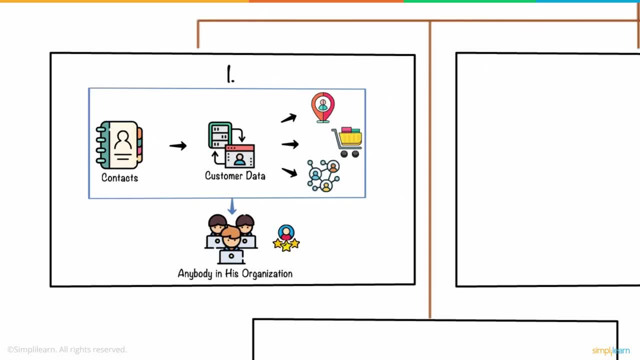 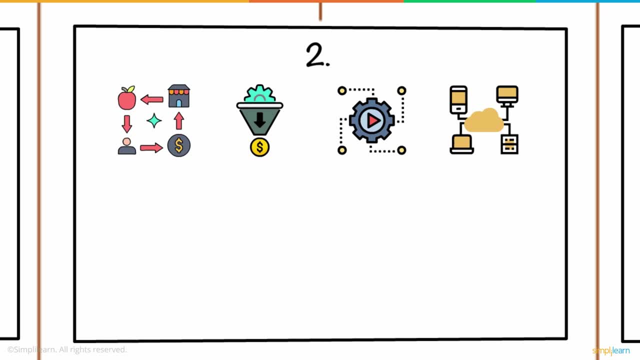 2. All data that Kevin has has a very precise control of all customer information. Even if he짓s the best part of his life, he can easily use it well. 3. All data is taken after a very specific question created in a CRM database. fighter: 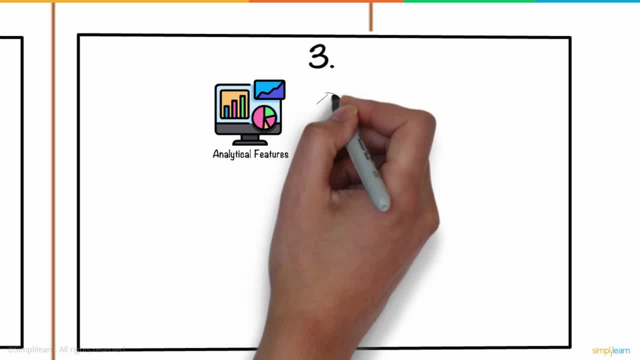 As a whole. it automatically tied on different parts of the designers background, even in the settings themselves. These are primarily used for its sending behavior and execution technologies, such as update settings, guiding data, matching the surtout of media and, finally, coordinating a head Start using our every time pyramid. 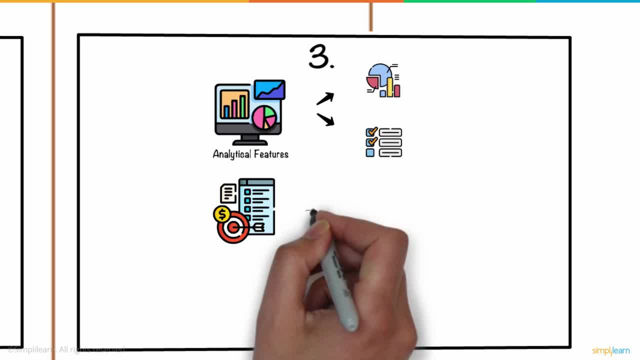 Everyone is care about improvement at thelaughter desk when you need to implement CRM, that's all in your data store. Two: Kevin may assess the performance of a marketing strategy and adjust his optimization strategies using metrics like click-through rates, churn rate and demographic data. 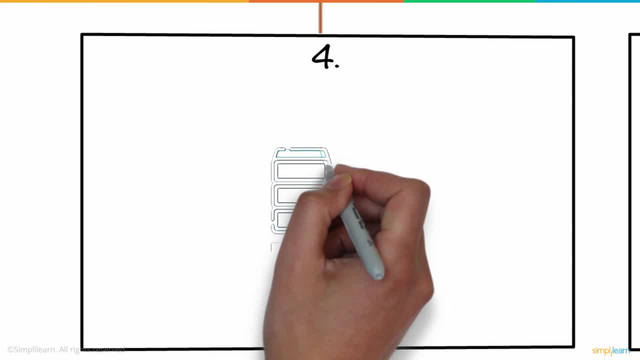 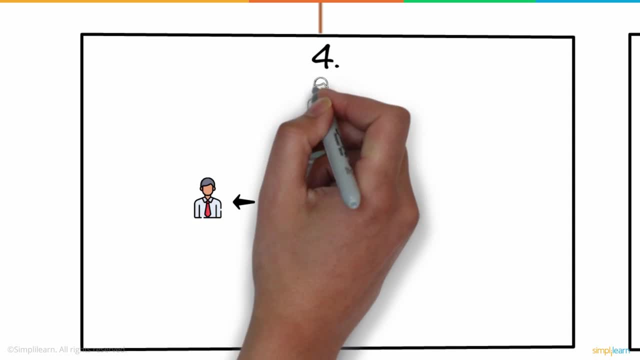 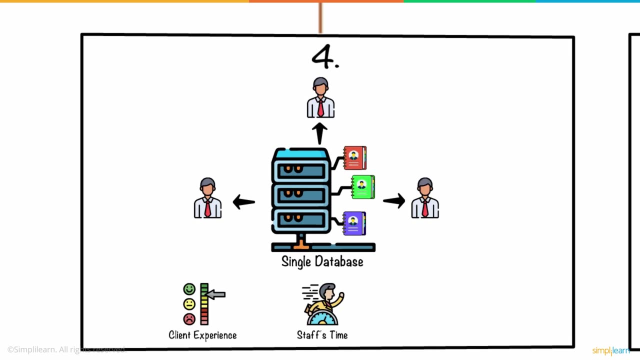 Four: one more thing that CRM software excels at is creating a single database that houses all of Kevin's company's client information and makes it readily available to anyone who needs it. This improves and increases the client experience, while saving his staff time from having to go through outdated files and information. 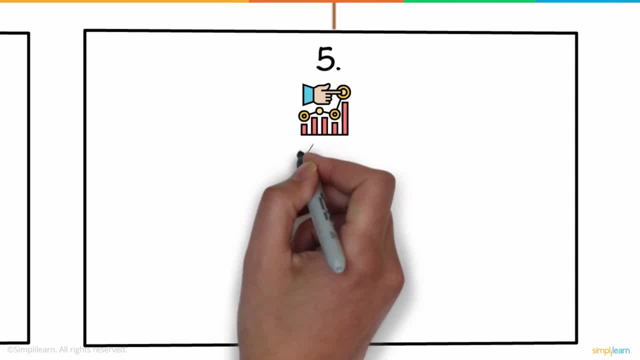 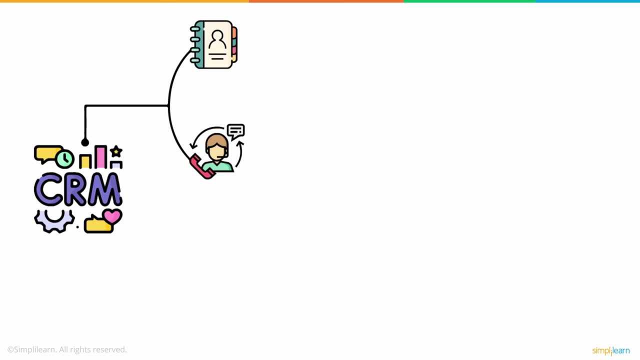 Five, Kevin may see important trends and gain a sense of what to anticipate from his future sales cycle performance. with the automated sales reports and CRM software, He can then modify its goals and targets to fit these estimates. CRMs automate operations like contact, communication and collaboration. 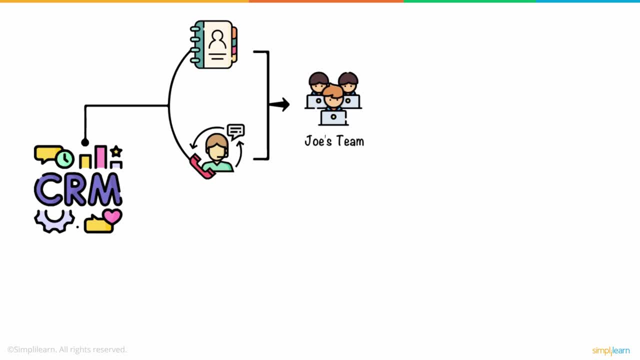 So Joe's team's daily tasks and procedures will move much more quickly. thanks to the software. The CRM can also minimize mistakes and guarantee that all communications are sent to the appropriate recipients at the appropriate times. Thanks to Kevin's guidance, Joe can now focus on the important aspects of running a business. 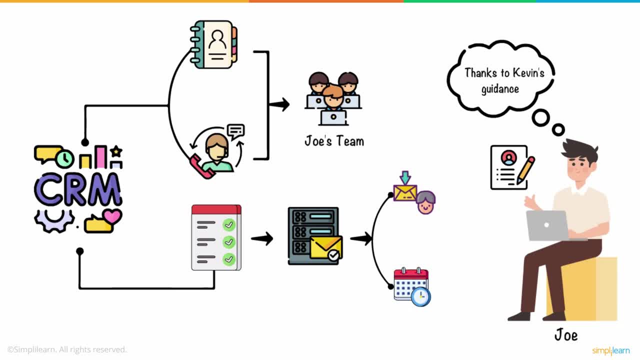 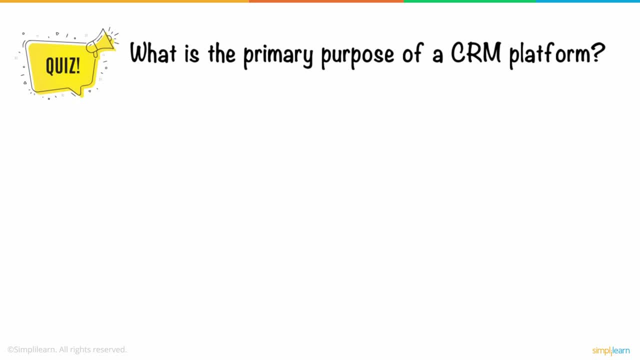 rather than manage the nitty-gritty details on a logistical level. So here's a question for you: What is the primary purpose of a CRM platform? One: finding leads for business acquisition. Two: maximizing revenue through lead and resource management. Three: help create multiple income streams for an organization. 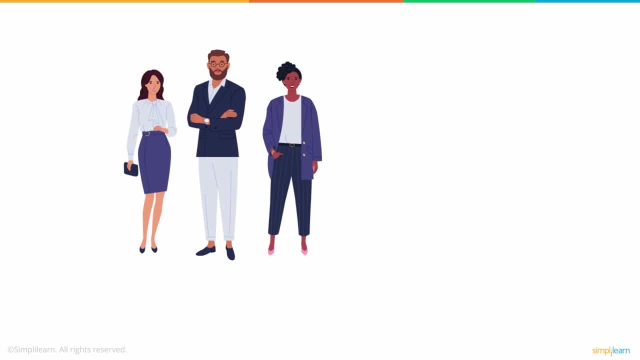 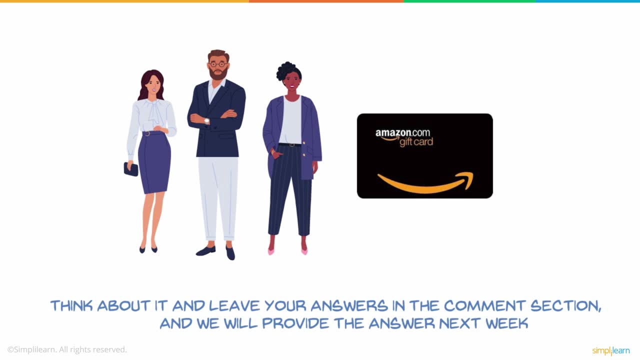 Give the correct answer, along with your reasoning, and stand a chance to win an Amazon voucher. Think about it and leave your answers in the comment section, and we will provide the answer next week. We hope you enjoyed this video. If you did, a thumbs up would be really appreciated.